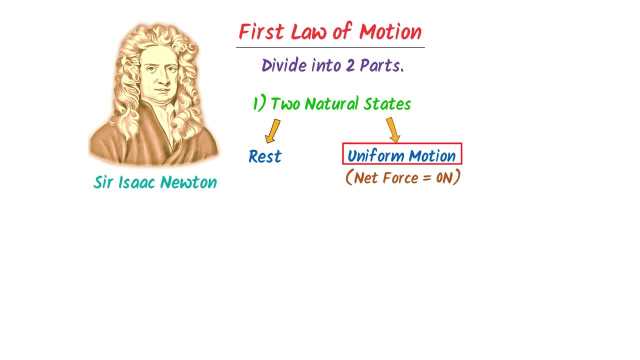 we say that F is equal to zero. Now consider this ball at the rest. According to Newton-Baba, state of rest is the natural state of the ball. Secondly, consider this car. Let this car is moving in a straight line with uniform speed. According to Newton-Baba, this uniform speed 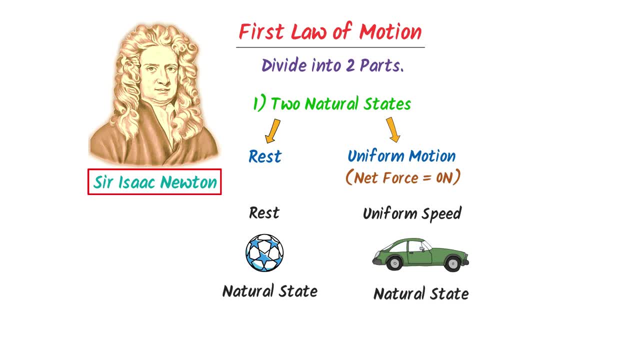 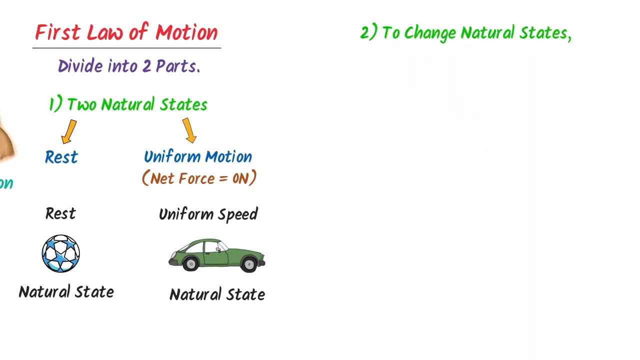 or uniform motion of this car is also natural state. Secondly, Newton-Baba states that if you want to change natural state of any object, you need external force or unbalanced force. For example, consider the ball at the rest. When you kick this ball, you exert external force on. 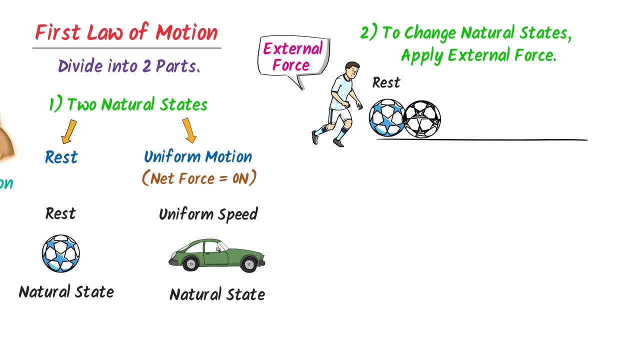 the ball. As a result of this, you change the state of rest and the ball starts moving. After covering some distance, the ball will stop Here. let me ask you: what is stopping the ball? Well, the answer is simple: The friction force of the ground is stopping the ball. 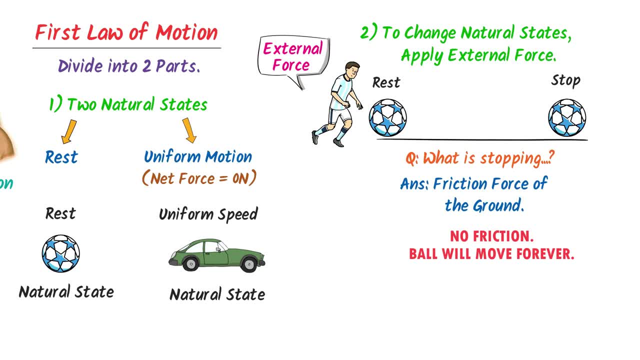 If we eliminate the friction force of the ground, the ball will stop. If we eliminate the friction force of the ground, the ball will continue its state of motion forever. Secondly, consider this moving car. When you suddenly apply brakes, you exert force on the. 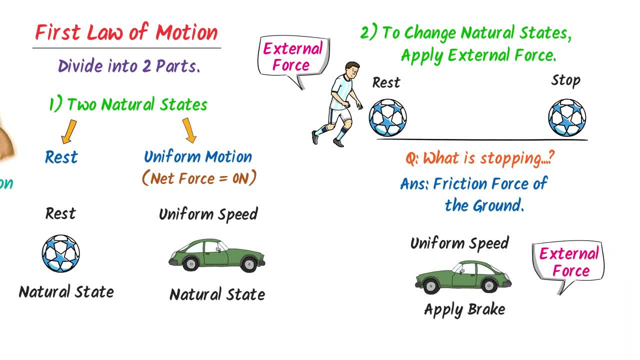 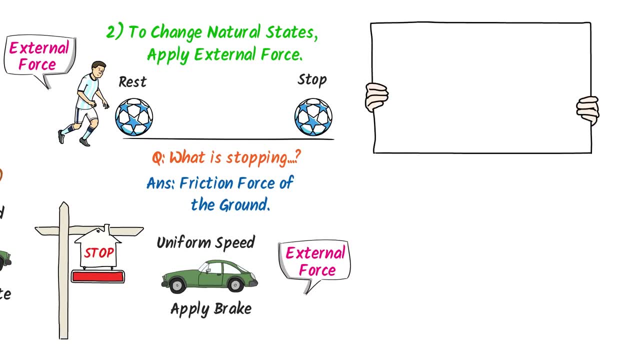 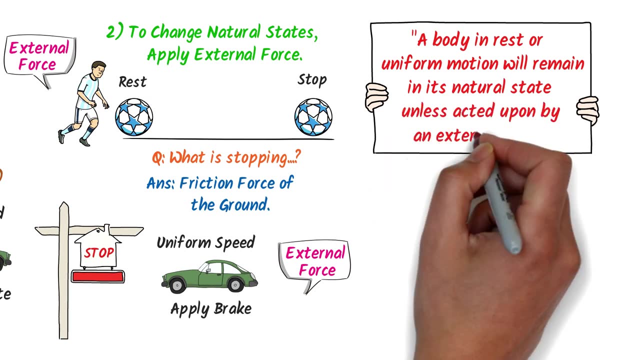 car and you change the state of uniform motion of the car. As a result of this, the car stops. Therefore, Newton-Baba states that a body in rest or uniform motion will remain in its natural state unless acted upon. In fact, Newton-Baba states that a body in rest or uniform motion will remain in its natural state. 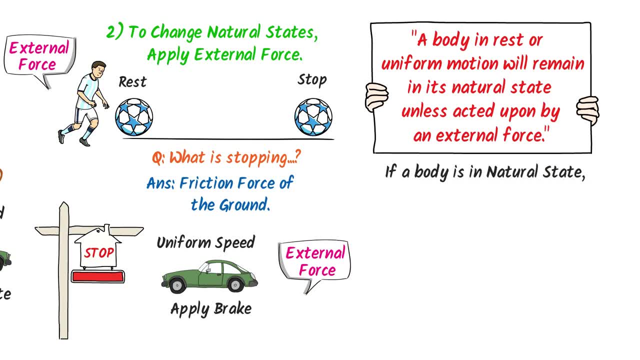 unless acted upon. Remember that if a body is in natural state, the net force on the body is always equal to zero. Some very talented people and very famous book write: F is equal to zero. Personally, I do not like this. I always write: net force is equal to zero. Secondly, we can also say that if net force 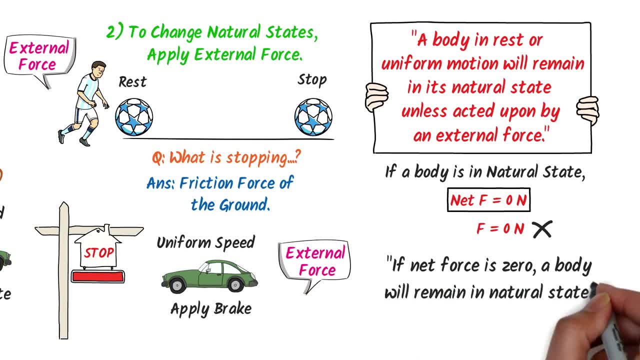 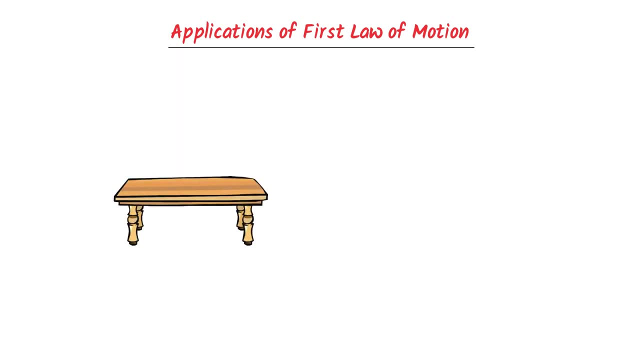 on a body is zero, a body will remain in its natural state. Therefore, we can also say that if net force on a body is zero, a body will remain in its natural state. Now let me teach you the application of Newton's first law in everyday life. Consider some books. 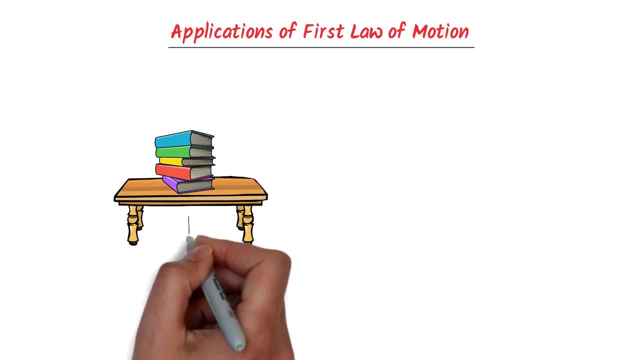 present on the table. We know that these books are experiencing the downward force of the gravity. Let this is 10 Newton force. At the same time, the table is exerting upward force on the books. Let this is also 10 Newton force. Now let me ask you: what about the net force on the books? 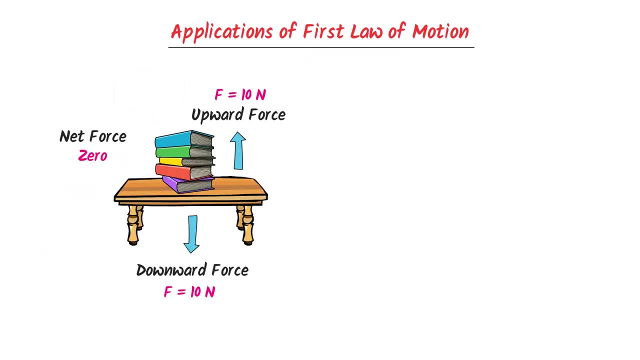 Well, the net force on the books is zero. So we say that these books are at rest, which is the natural state of the books. Secondly, consider the jumping of a paratrooper. We know that this person is experiencing the downward force of the earth. Let the downward force on this person is 500 Newton. 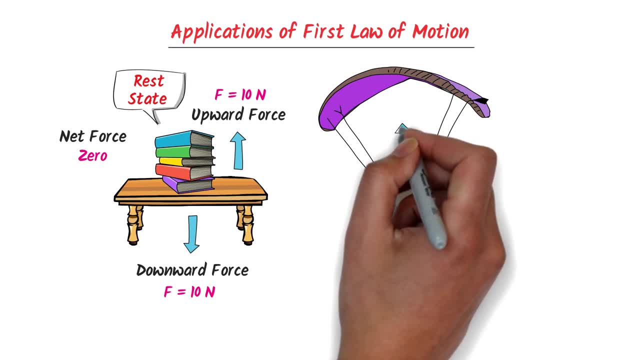 Let this is also 10 Newton force. At the same time, the table is exerting downward force on the books. Also, we know that at the same time, the air resistance is pulling this person in upward direction. Let this upward force is also 500 Newton. Now let me ask you, what about the net? 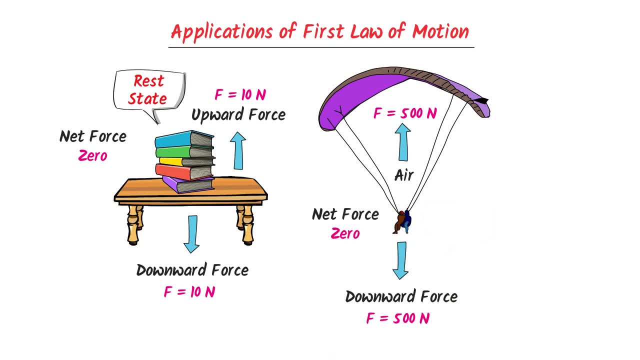 force. Well, the net force is zero, Newton. But we know that this person is still in uniform motion or it is moving with uniform speed towards the earth. Here a lot of students are confused. They think that if the net force is zero, then why the paratrooper is moving with uniform speed. 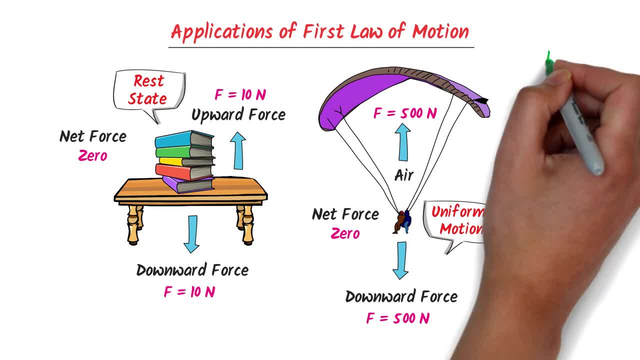 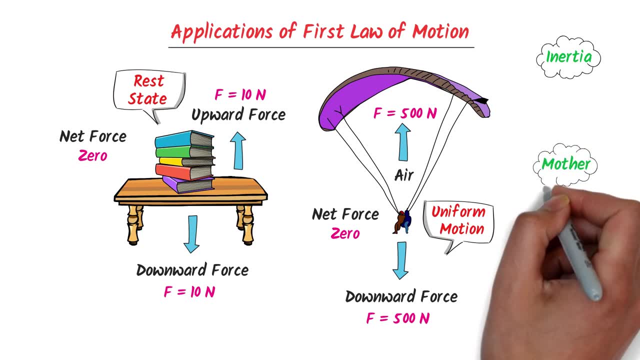 towards the earth. Well, the answer is simple: It is due to inertia. If you want to understand inertia, I always connect it with the mother. We know that every mother care about her children and she want to keep their children in good health. Similarly, inertia always want to keep. 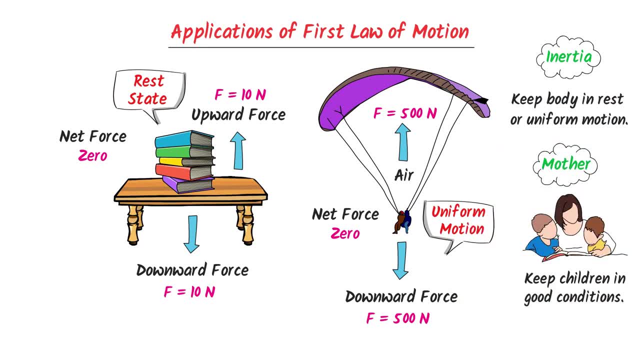 the body in its state of rest or in its state of uniform motion. One can also say that inertia tends to keep the body in its initial position of rest or initial position of uniform motion. For instance, initially the paratrooper was moving in downward direction. Even the net force. 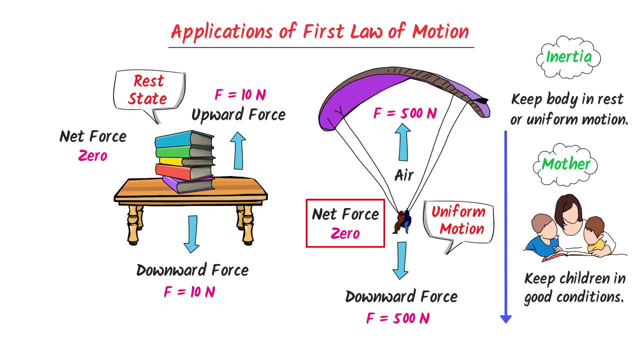 on the paratrooper is zero, but inertia tends to keep its uniform motion in downward direction. Remember that if a body is at rest, the net force is always zero. Secondly, if an object is in uniform motion, the net force is again zero. So in Newton's first law of motion, 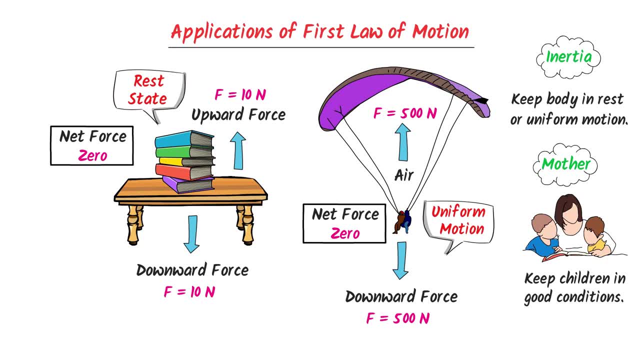 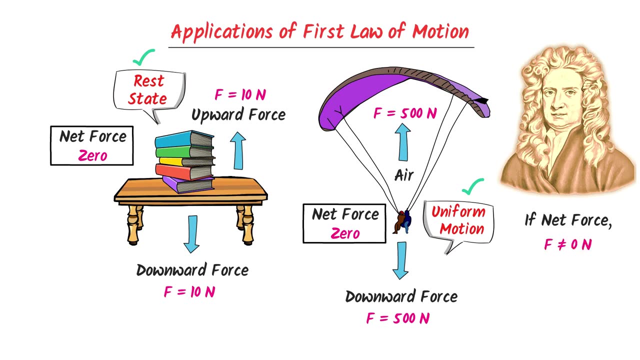 we learn that there are two states of any object. The first one is the state of rest and the second one is the state of uniform motion. Now here, Newton's baba thought that what would happen if the net force on an object is not zero? To answer this question, Newton-Baba. 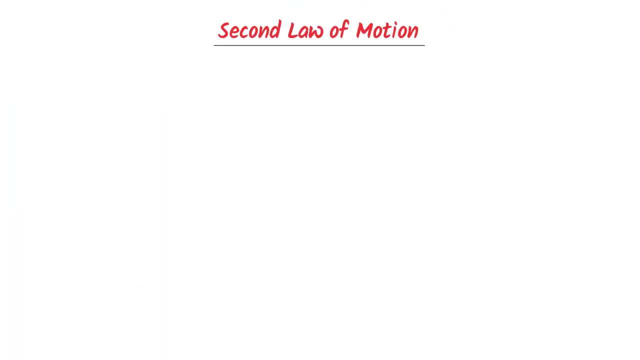 presented his second law of motion. We know that if the ball is in the rest, it is its natural state and the net force on the ball will always be equal to zero. Secondly, if the car is in uniform motion, it is also its natural state and the net force on the car 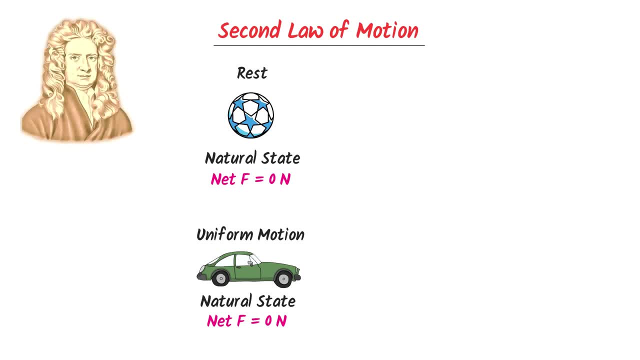 will also be equal to zero. Now Newton-Baba states that if we exert force on this stationary ball, force will change its velocity. For example, initially the velocity of the ball was zero. After exerting some sort of force on it, let its velocity change to 5 m per. 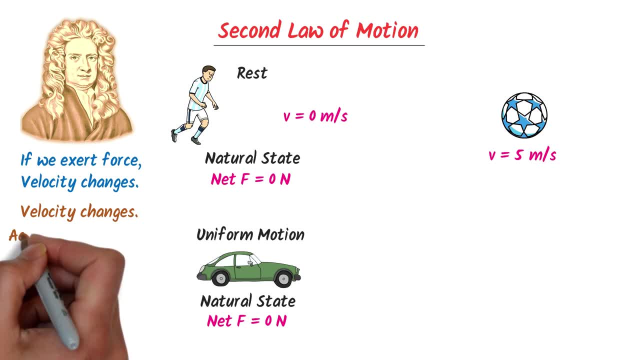 second, We know that when velocity changes, acceleration produces, So indirectly. Newton-Baba states that when net force is not equal to zero, it produces acceleration. Let me repeat it: When net force is not equal to zero, it produces acceleration. Secondly, when we suddenly 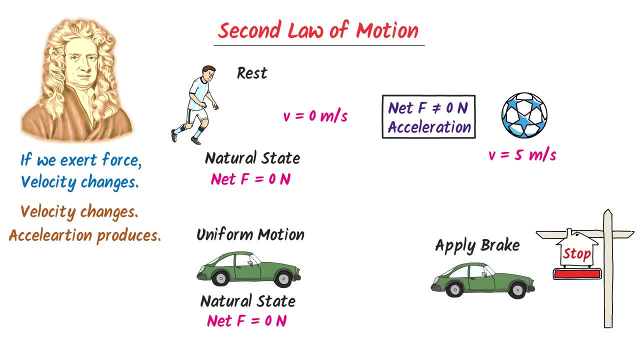 apply brake, we exert force and the car comes to rest Again. Newton-Baba states that force changes velocity of the car. For example, let the initial velocity of the car go 1 m per second. We know that if the ball is in uniform motion, it is its natural state. 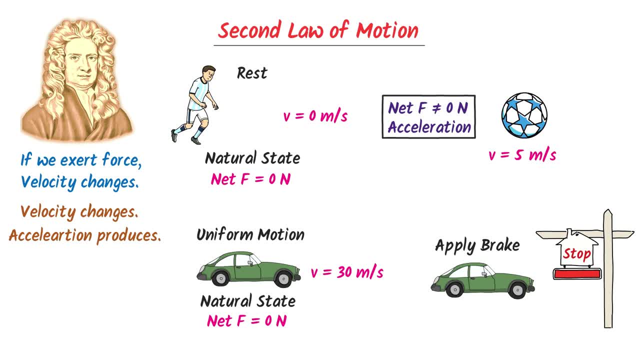 and the net force on this stationary ball will always be. its natural state After exerting was 30 m per second. after exerting some sort of force, the velocity of the car is zero because it has stopped Here. velocity is changed. We know that when velocity changes. 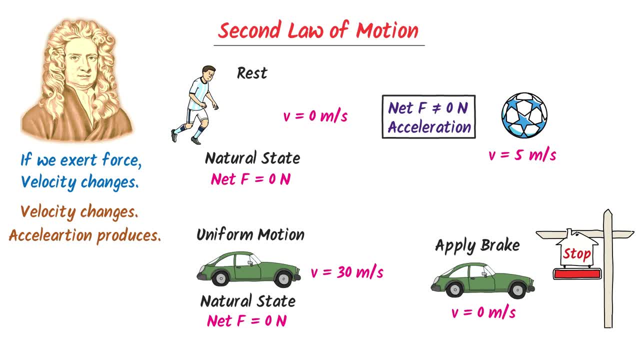 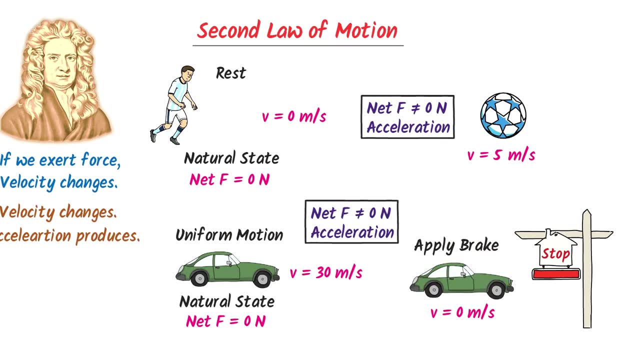 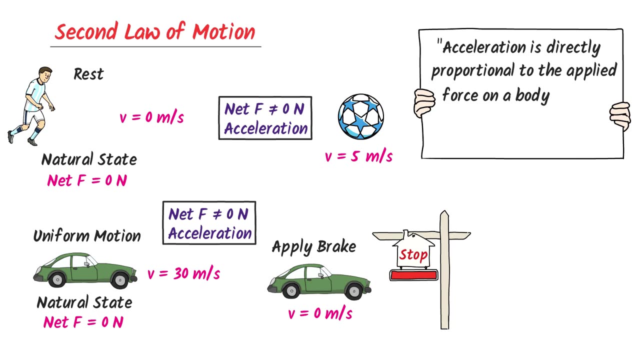 acceleration produces So indirectly. Newton-Baba states that when net force is not equal to zero, it produces acceleration. Therefore, acceleration is directly proportional to the applied force on a body. Secondly, he states that acceleration is inversely proportional to the mass of a body. Or we write: F is equal to ma, For example. consider this car and. 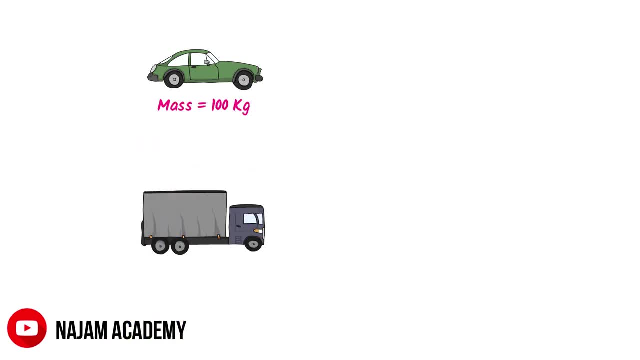 this truck. Let the mass of this car is 100 kg and the mass of this truck is 200 kg. Let I exert 200 Newton force on this car and I also exert 200 Newton force on this car. Let I exert 200 Newton force on this car and I also exert 200 Newton force on this truck. 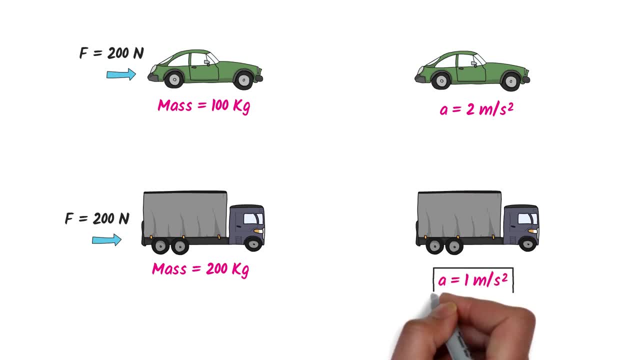 We would observe that the car will start moving with acceleration of 2 m per second square and the truck will start moving with acceleration of 1 m per second square. Here the truck is moving with acceleration of 1 m per second square because truck is 2 times heavier than 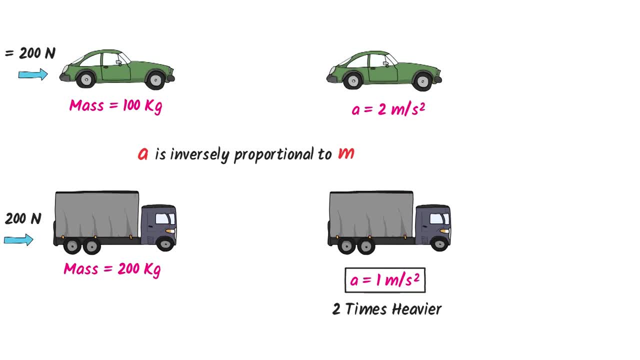 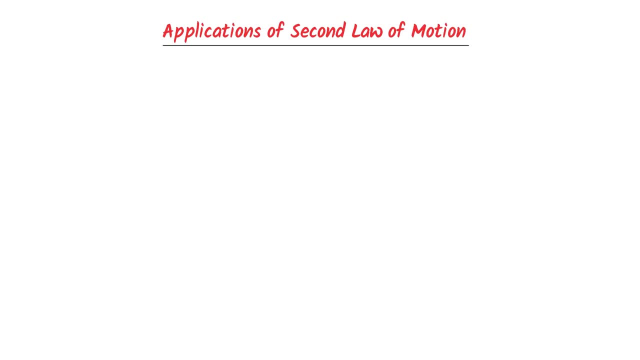 the car. So that's why we say that acceleration is inversely proportional to the mass of an object. important points of Newton's second law. Now let me teach you the applications of Newton's second law of motion in daily life. Remember that every accelerated object is explained. 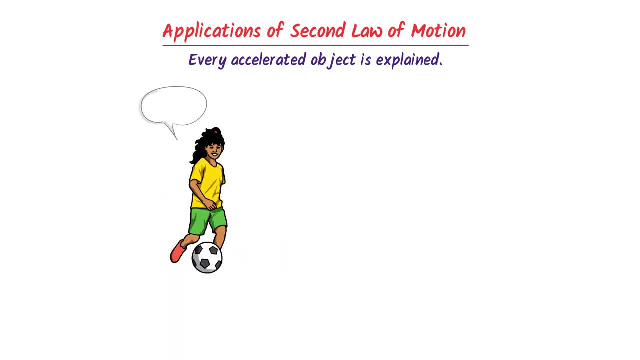 by Newton's second law of motion. For example, when you kick a ball, you exert force on it and the ball is accelerated in the direction of applied force. Secondly, when we push accelerator of the car, we exert more force on the car body As a result of this acceleration or speed of the 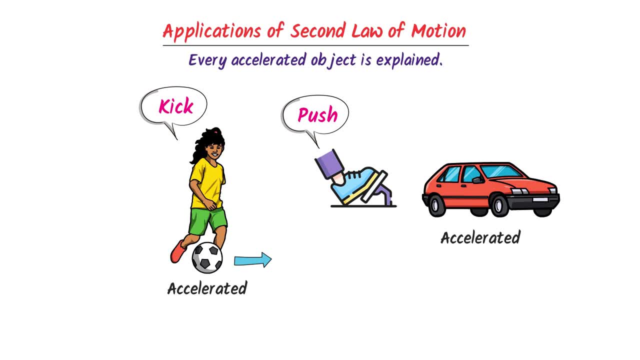 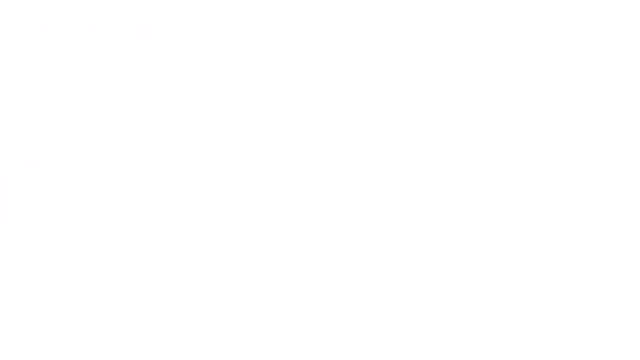 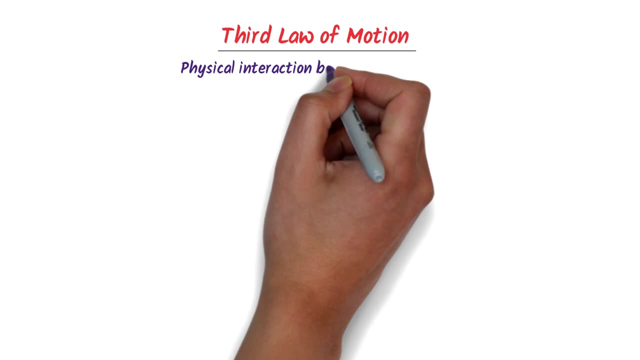 car is increased. Thus, remember that every accelerated object is explained by the help of Newton's second law of motion. Now, what about Newton's third law of motion? Remember that Newton's third law of motion is all about physical interaction between two objects. For example,